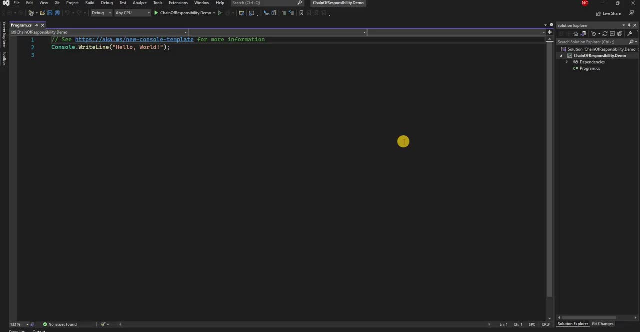 chain of responsibility design pattern. I am going to consider an expense report approval scenario. So basically, we will have three levels of approval and when an expense report is created it will go through three levels of approval and each approval level you can consider as a handler and then the handler. each handler will propagate to the next handler. 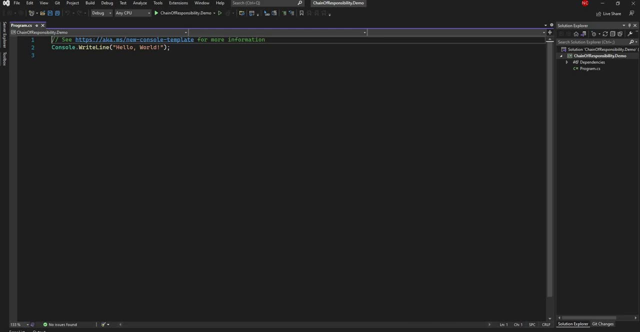 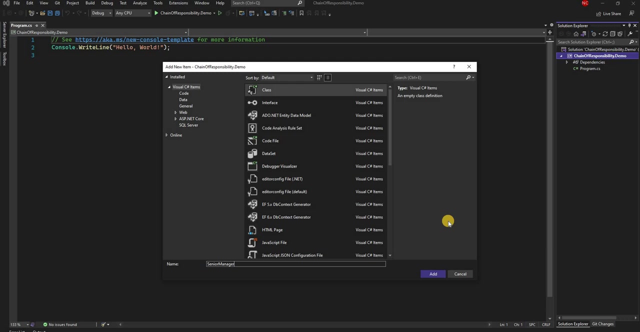 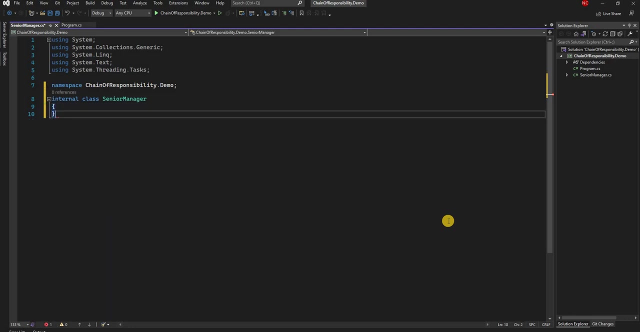 to handle the request. That way we create a chain of responsibility, as the name suggests. So for that first I am going to create a class for manager, who is the first level of handler or first one responsible for approval in the chain of responsibility. So I'm going to create a new class and I call it as SeniorManager and the SeniorManager. 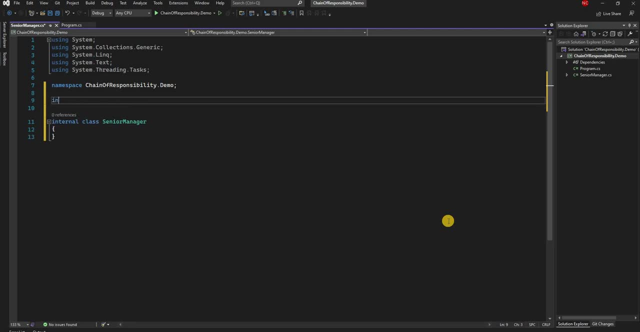 is going to implement an interface. Let me declare the interface here as well, and we're going to name the interface as IManager and the IManager, if you think about it, because this is a chain. and what is the main responsibility? The main responsibility is to approve an expense report. 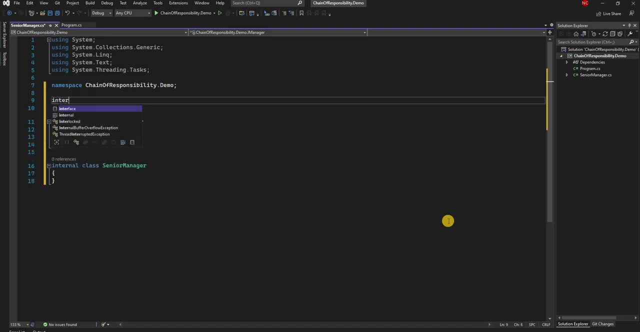 So first let's create the class for expense and we can create InternalRecordExpenseExpenseReport and the report is going to have a name. it will have other things also, but for simplicity I'm just keeping name. and the next thing is an amount: Amount. ideally should be double, but for this example I'm just keeping it as an integer. 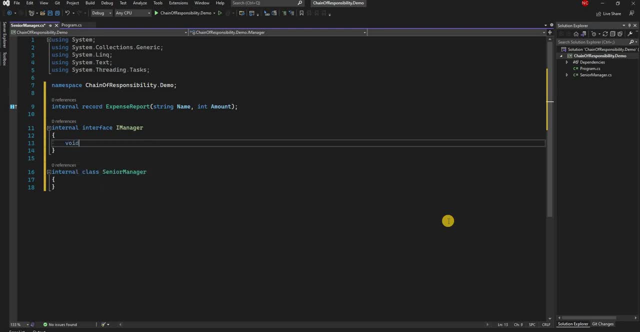 So the first thing the manager has to do is approve, so you can have approveRequest and it will take expenseReport as the parameter And also for a manager. The manager needs to know who is the supervisor or the next level in the chain of responsibility. 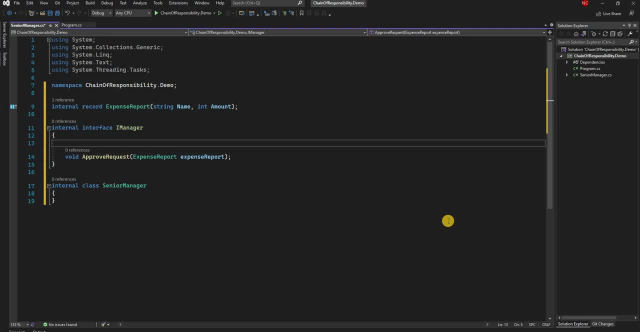 who will the approval fall back to if this manager is not able to approve? So for that we can create a method called void setSupervisor, and it is going to take IManager, because everyone is going to be a manager. So first one is SeniorManager. 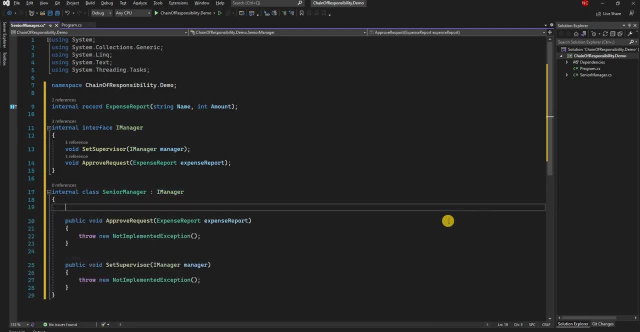 And let's implement IManager, and here we can create private IManagerManager and in this place we can say: manager is equal to thismanager is equal to manager. And in this case, what we are going to do is we're going to have a simple logic. we're going 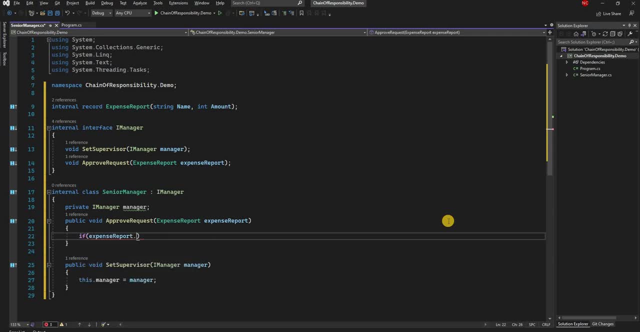 to say: if expenseReportamount is less than 500. Then we're going to have a simple logic. We're going to say: if expenseReportamount is less than 500. Then the manager can approve. And for the approval we're just going to have a consoleWriteLine and we can say approveByManager. 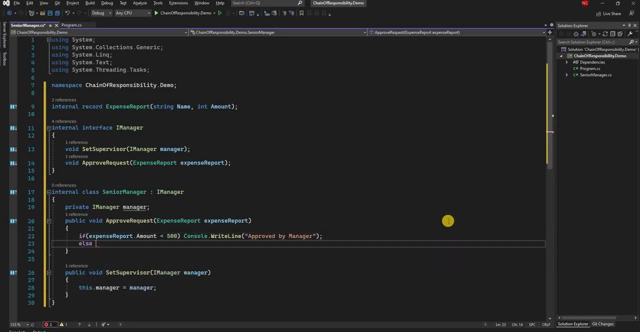 Else, what we are going to do is, if it is more than 500, then we are going to say else: ManagerApproveRequest, because then the SeniorManager is going to give it to the next level For approval And then after SeniorManager we're going to have another class, and I'm going to just create 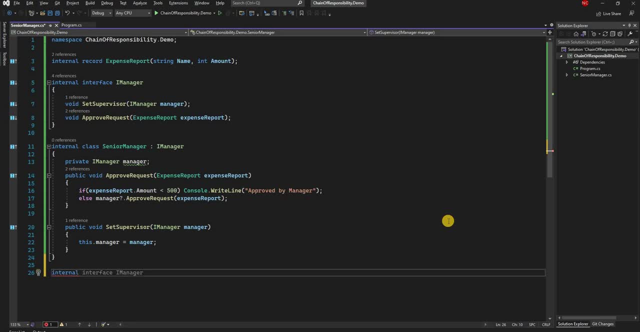 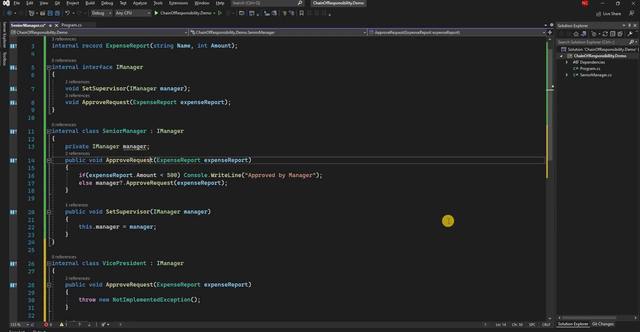 all the classes here, just for simplicity. but you can keep the classes into their own different file. You can create another class called VicePresident. It's also going to implement IManager and let's implement IManager, And here Similar to the SeniorManager. 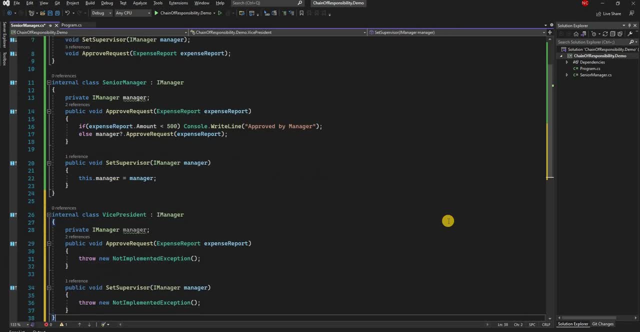 The VicePresident also is going to have the PrivateManager, and here we can say: thisManager is equal to Manager And here for the VicePresident we are going to: the amount that VicePresident can approve is up till 1000.. So you can say: 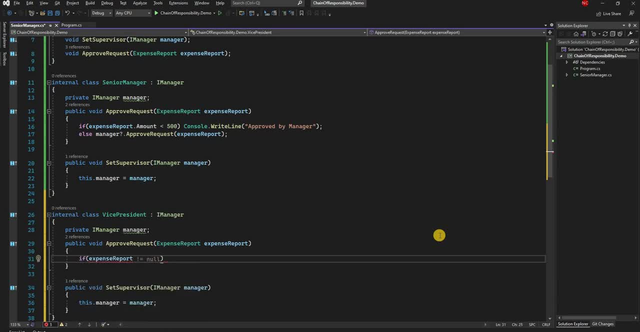 If ExpenseReportAmount is less than 1000, then again let's do a ConsoleWriteLine and here we can say approvedByVP- Else. If that's not the case, then ManagerApproveRequestAmount: ExpenseReportAmount- ExpenseReportAmount. 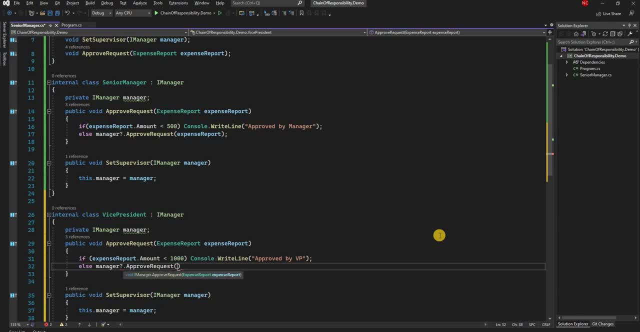 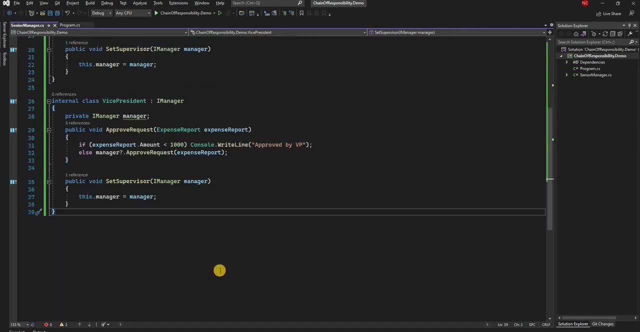 ExpenseReportAmount, Then it is just sending it to the next level, And then, finally, we will have the third class, which is going to be InternalClassCEO, And let's say that's the last level. And here, similarly, we're going to have PrivateManagerAdmin. 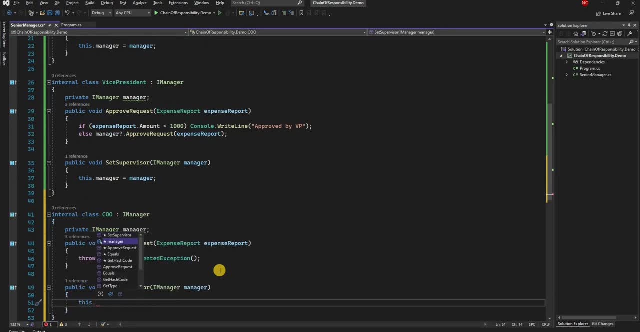 private manager set this dot manager is equal to manager. and here we can say: co can approve up till five thousand dollar. so if expense report dot amount is less than five thousand dollar, then ceo is just going to go ahead and approve it. otherwise, in this case, ceo is just going to say not approved. 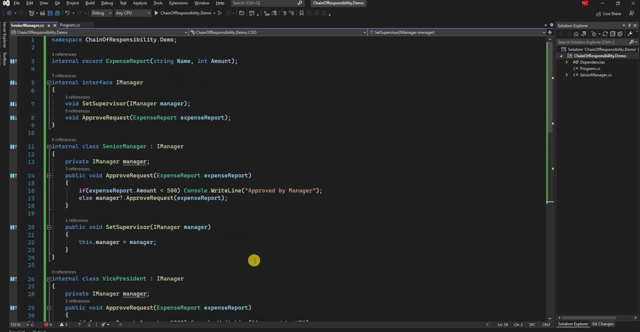 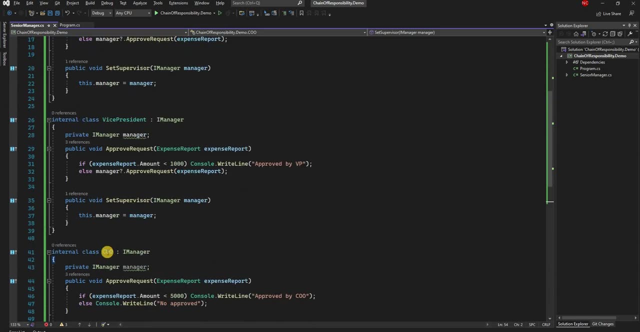 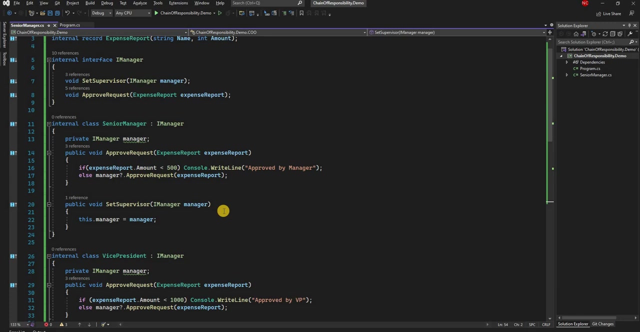 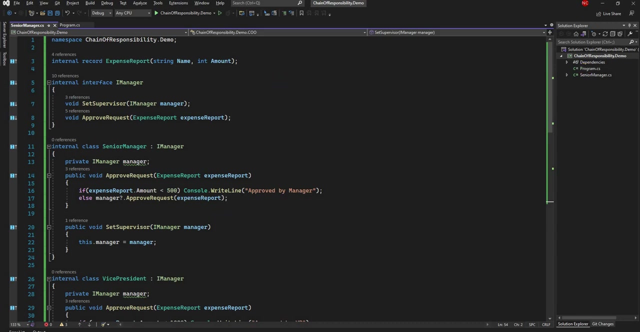 so that's how we created three different hierarchy, but without creating uh inheritance. so senior manager, vice president, as well as ceo, all are implementing imanager, but they have their own supervisor and, based on a situation, the responsibility will go to the next one in the chain, and that's a classic implementation of chain of responsibility. 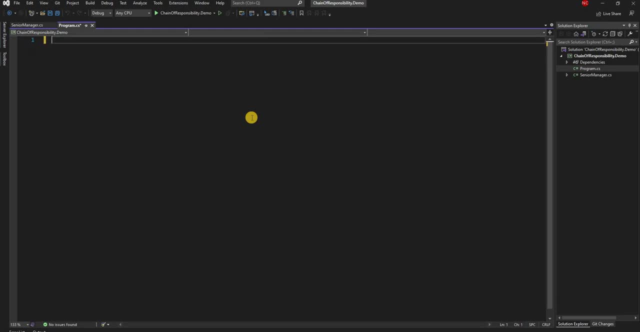 and then what we can do is we can go here and we can say: var manager is equal to new senior manager, let's add the namespace. and then we can say: var dp equal to new vice president and finally, var co equal to new c ceo, and then we are going to set the supervisor. so for manager, the supervisor is going to be vp. 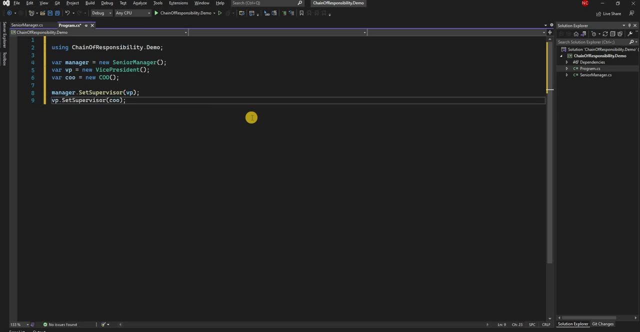 for vp supervisor is going to be ceo. and now let's create a. let's create an expense report. expense report, and let's say: we're buying a monitor, it's going to cost 100, and then we can just have console dot right line of expense so that we print. 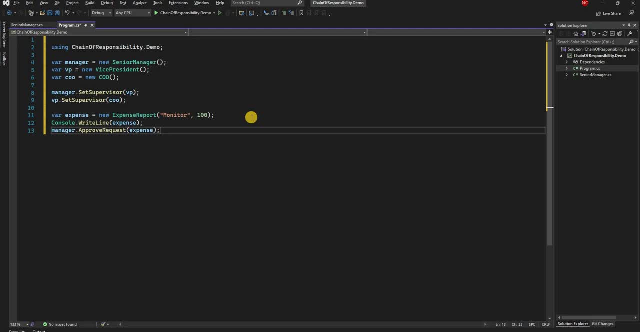 out what it is and then let's do manager dot. then, similarly, we are going to have two more expenses. the next one, let's say it's going to be a desk, because we all are working remotely stays. it's going to cost $900. and the third one is going to be, let's say, a travel expense, and it's 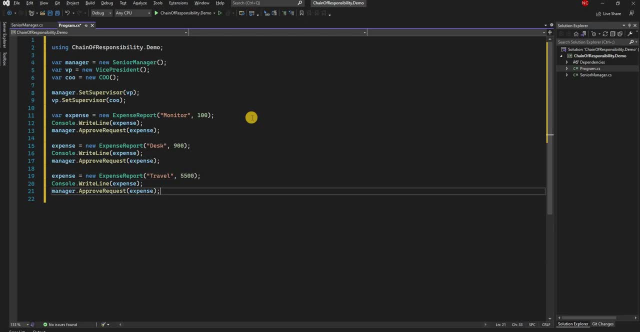 going to cost $5,500, and then we're just going to see in the chain which handler handles the response, and I can just add a delineator here just for better readability in the console. okay, now let's run this application, and in the future we will be able to run this application in the. 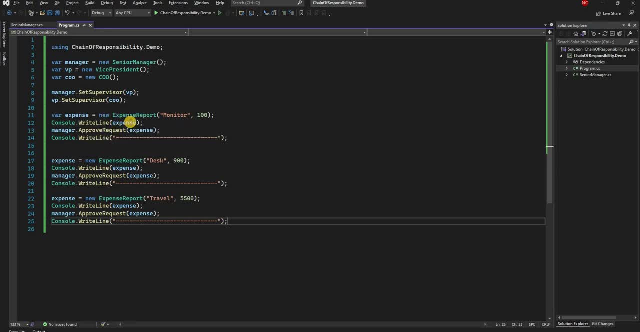 future. we will be able to run this application in the future. we will be able. first case: we should see that the senior manager itself is able to approve. in the second case, it is going to go to the VP and VP is going to approve. in the third case is going to go to the CEO, but CEO is going to decline because it is. 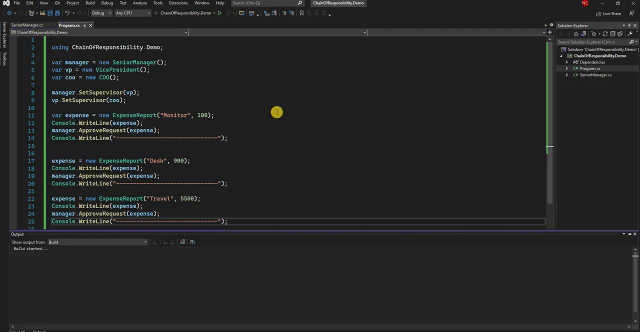 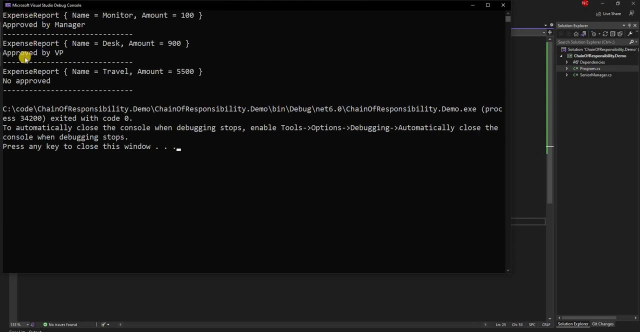 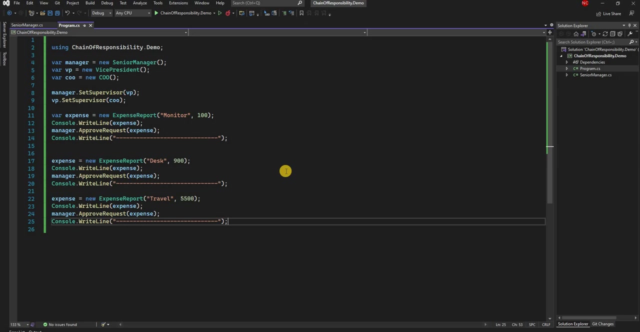 even beyond the amount the CEO can approve. so let's run this and once we run, we can see that the first one is approved by manager, second one is approved by VP and the third one is not approved, as expected. So this is, in essence, very simple implementation of chain of responsibility design. 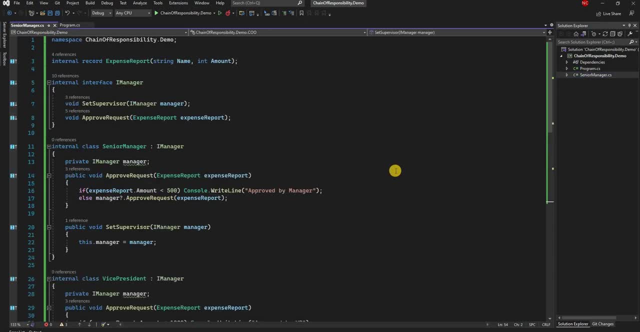 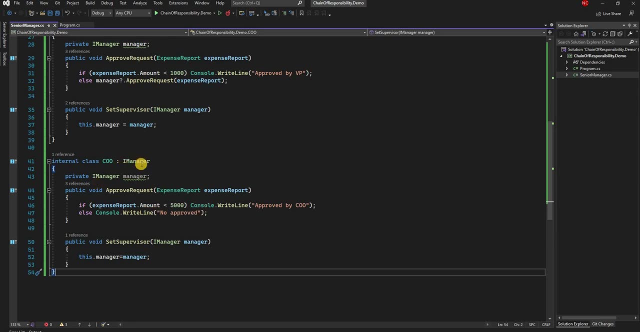 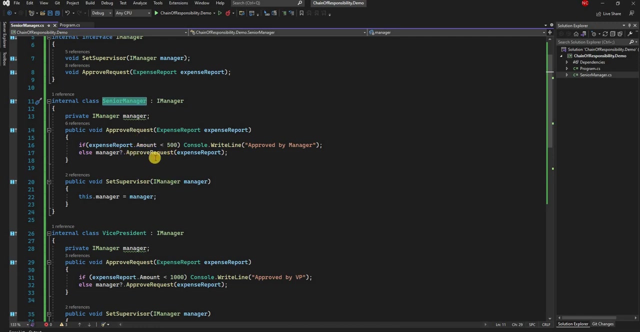 pattern. Now, one thing about chain of responsibility design pattern. as you can see, this is something which complements the solid design principles because, as you can see, we are still using a single responsibility principle, where we are deciding which manager can approve what amount, but then we are adding the supervisor concept, using which we are adding the next handler. 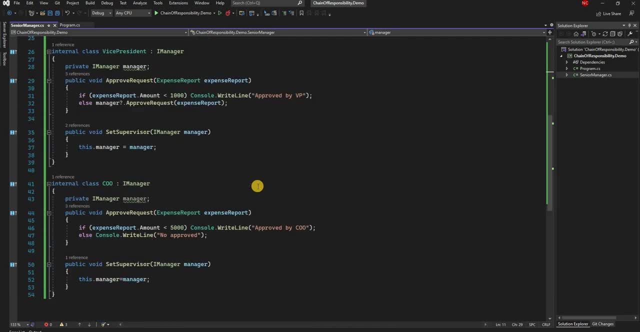 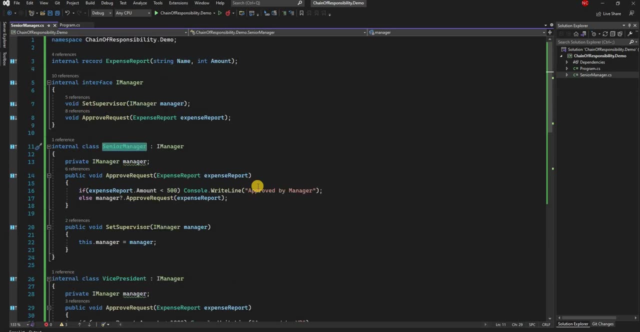 in the pipeline for the request to go, and this is how we can create a chain of responsibility principle. So that is all I wanted to cover for today's video. If you like this video, please give me a thumbs up If you are new to my channel and you think you are getting well out of my channel. 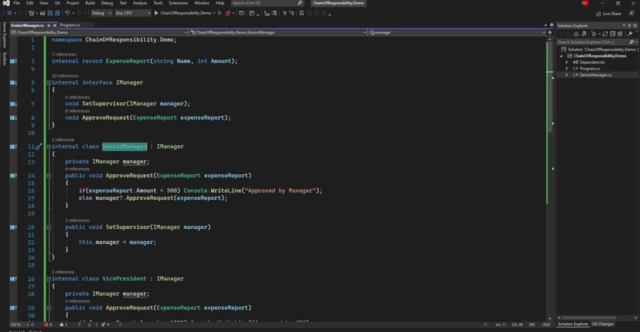 please subscribe to my channel and thanks so much for watching this video.